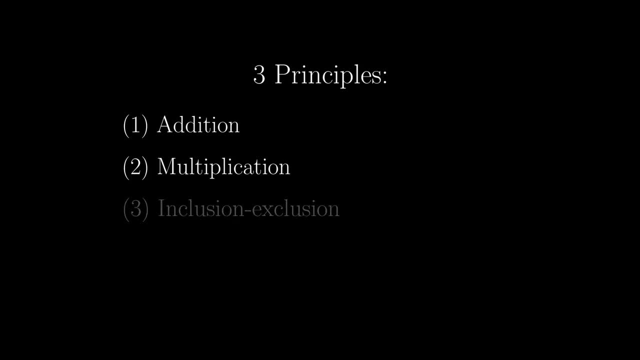 this video series. we would rarely use any tools based on the inclusion-exclusion principle, but for the sake of completeness I would also include it in this series. Some might remember permutations, Permutation and combination as a symbol for combinatorics, but they are tools based off. 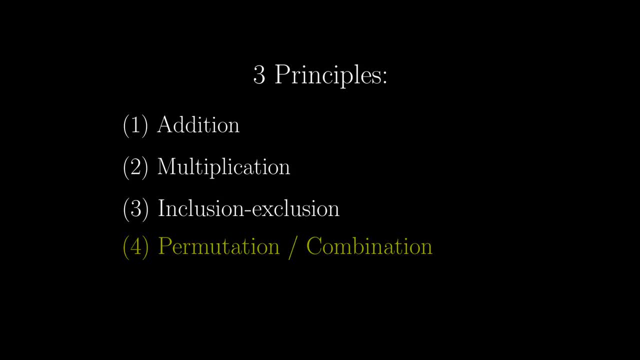 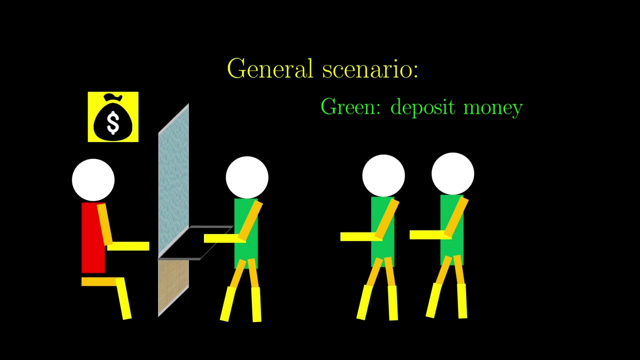 of the multiplication principle. So the founding principles are really just these three. The entire video series builds on one very general scenario. Let's say we are at a bank and people are queuing up either to deposit money denoted in green or to borrow. 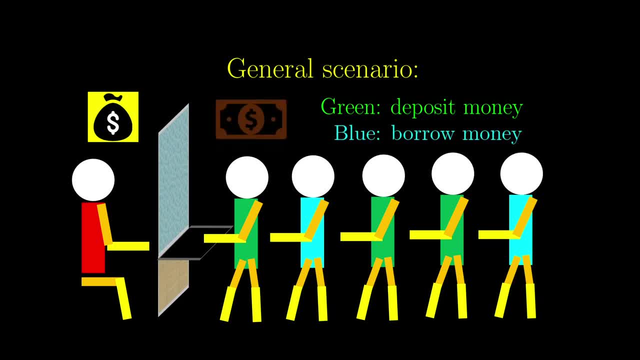 money denoted in blue Suppose. all transactions are in green Suppose. all transactions are in blue Suppose. all transactions are in blue Suppose. all transactions are done in cash. If the bank does not have enough cash to lend, the transaction is not successful. There are A number of people, each of whom deposits. 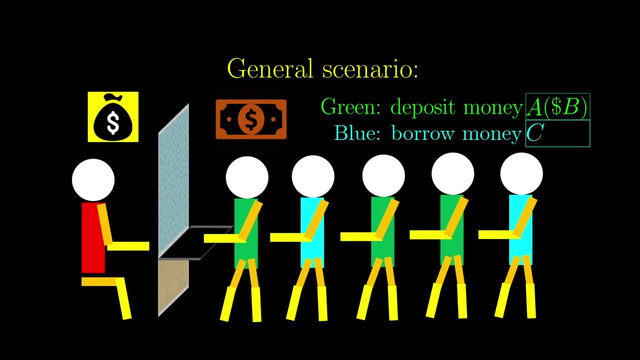 B dollars. On the other hand, C number of people all want to borrow D dollars. The bank originally has only E dollars of cash. Your job is to arrange these customers in a queue so that every transaction is done in cash. That means if at some point the bank does not have any cash, the next person in line 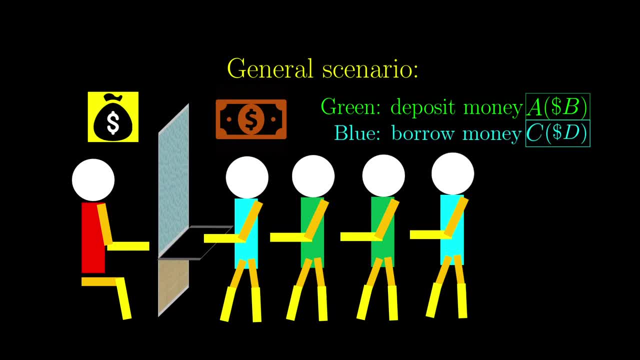 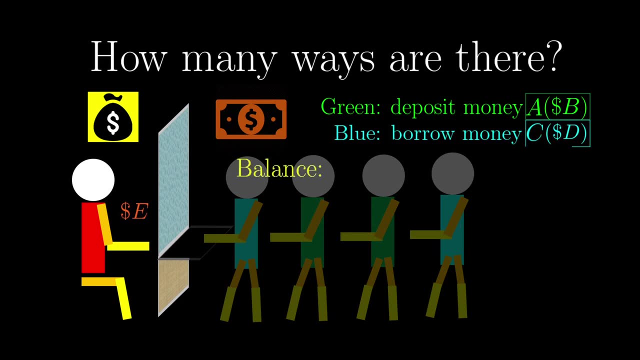 cannot be borrowing money. You should have prevented it from happening in the first place. The question is, under these constraints, how many ways there are to queue up these customers. There is something to note: The amount of money that the bank has after all those transactions. 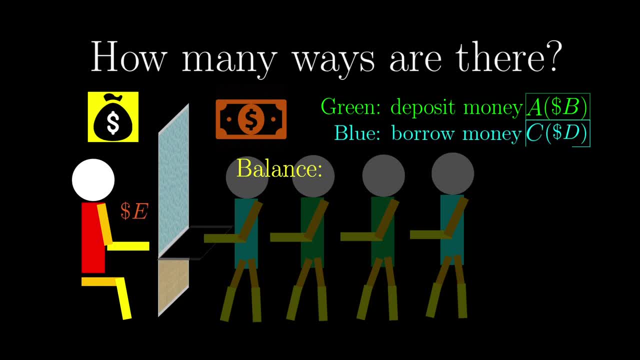 is independent of the arrangement. That is why there are so many ways to queue up customers, arrangement of the customers and the balance is given by AB plus E minus CD, where AB plus E is the amount gained and CD is the amount lost. This balance has to be non-negative. 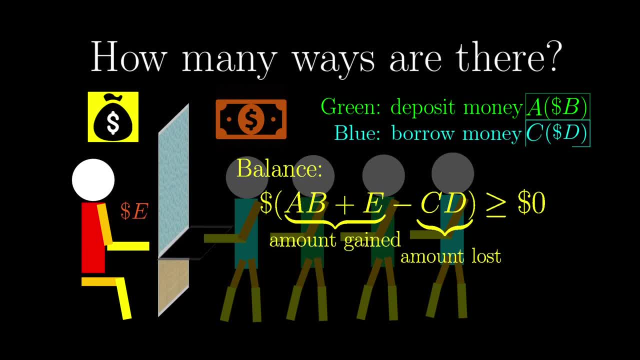 Otherwise, no matter how you arrange the customers, you can never make all transactions successful. As far as I know, the problem of how many ways there are to queue up the customers with so many variables is still unsolved. This shows how counting systematically can be difficult. 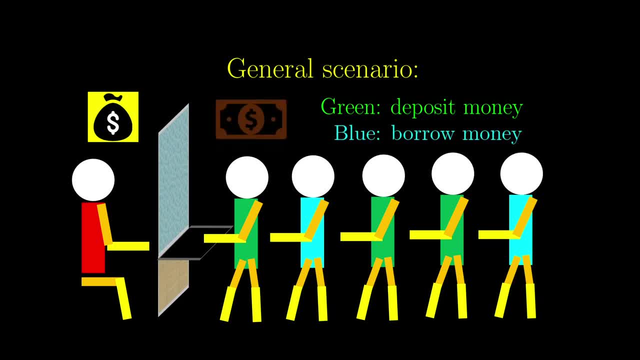 money denoted in blue Suppose. all transactions are in green Suppose. all transactions are in blue Suppose. all transactions are in blue Suppose. all transactions are done in cash. If the bank does not have enough cash to lend, the transaction is not successful. There are A number of people, each of whom deposits. 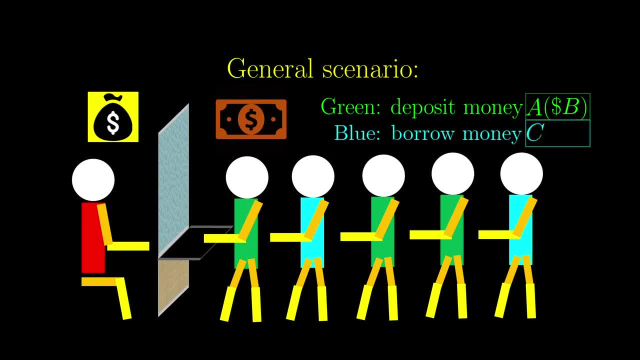 B dollars. On the other hand, C number of people all want to borrow D dollars. The bank originally has only E dollars of cash. Your job is to arrange these customers in a queue so that every transaction is done in cash. That means if at some point the bank does not have any cash, the next person in line 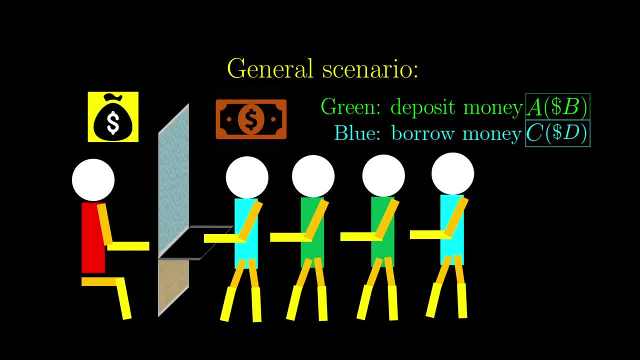 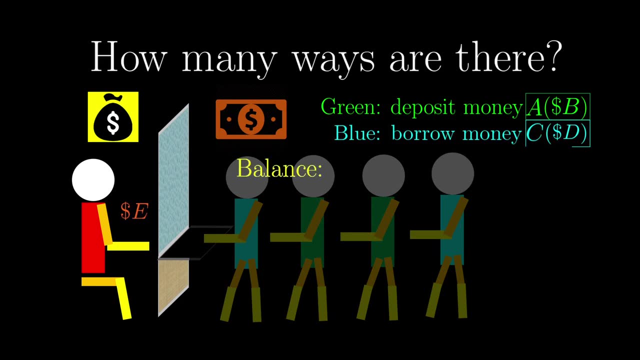 cannot be borrowing money. You should have prevented it from happening in the first place. The question is, under these constraints, how many ways there are to queue up these customers. There is something to note: The amount of money that the bank has after all those transactions. 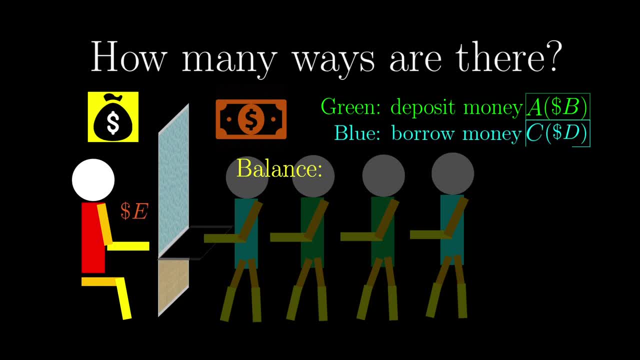 is independent of the arrangement. This is a very serious issue. The amount of money arrangement of the customers and the balance is given by AB plus E minus CD, where AB plus E is the amount gained and CD is the amount lost. This balance has to be non-negative. 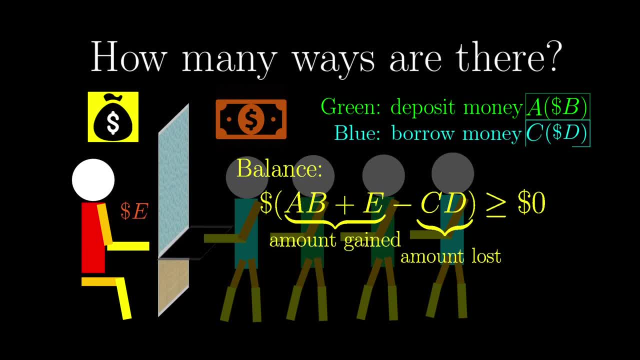 Otherwise, no matter how you arrange the customers, you can never make all transactions successful. As far as I know, the problem of how many ways there are to queue up the customers with so many variables is still unsolved. This shows how counting systematically can be difficult. 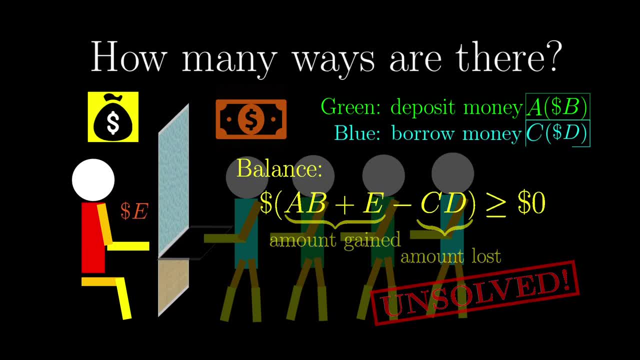 and, in this case, extremely difficult. However, if we have some constraints on the variables, like this one, then the problem can be solved. In fact, this particular constraint is the situation that we will discuss in the video after the next one. You might want to try the problem under this constraint before. 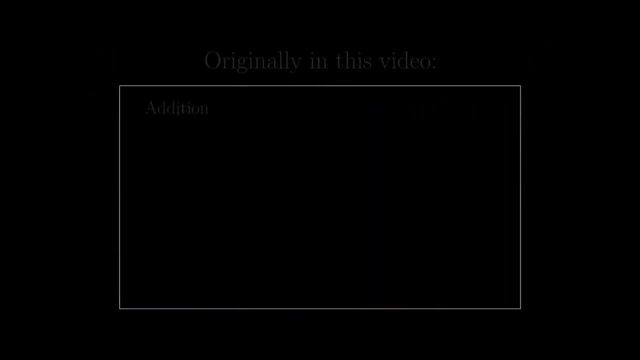 I review the video. Originally, I wanted to have a crash course in combinatorics in this video, but it turns out that this introductory video would then be too long. I would put it in the next video, though This is because I have previously asked viewers to fill in the Google Form linked.